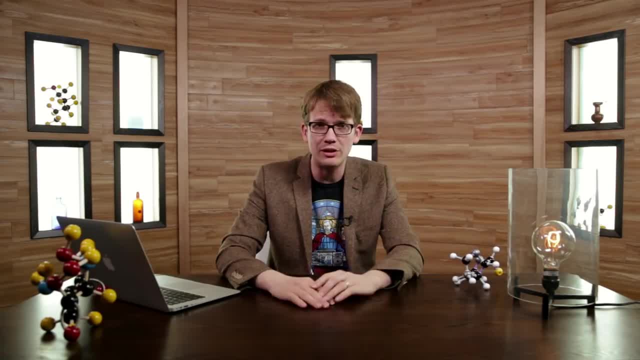 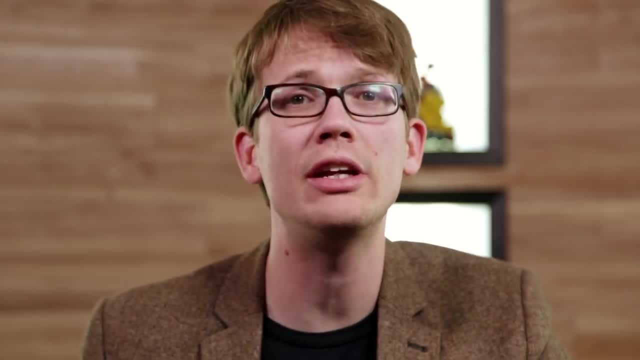 in reactions, and their numbers do change, huge amounts of energy can be released, far more than by the transfer of electrons that we've learned about in other reactions. When these changes happen to the nucleus of an atom, we rather logically call their study. 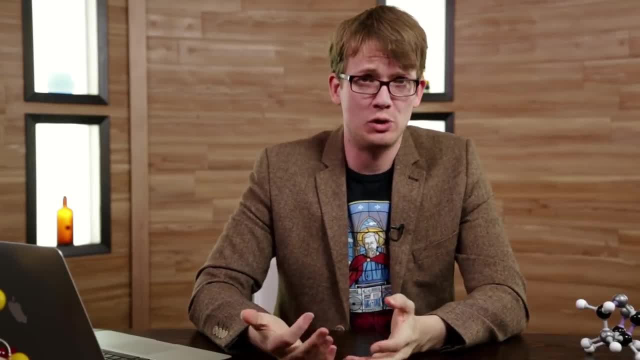 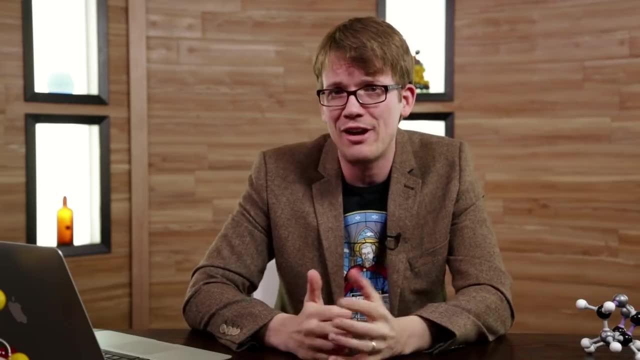 nuclear chemistry. Now, it's probably occurred to you already that changing the nucleus of an atom can completely change it's… nature. Protons are the key to an atom's identity, so any change that affects the number of protons will turn one element into a completely different one. An alchemist's dream, right. 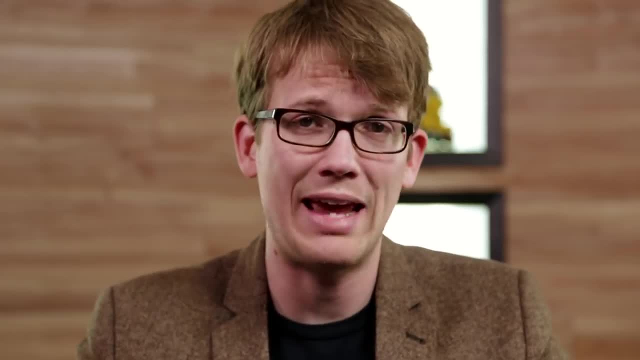 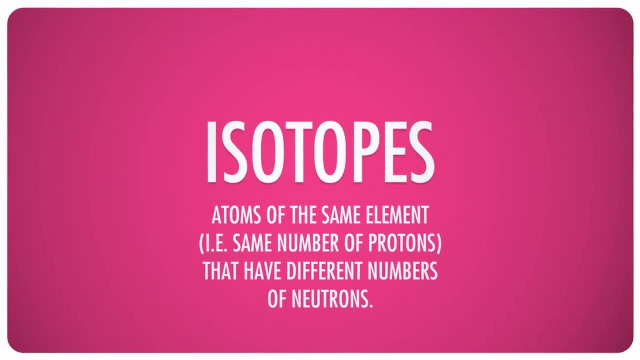 Lead to gold. So, as you might expect, that's not something that usually happens in a typical chemical reaction. The same can be said of that other component of the nucleus neutrons: Atoms of the same element that have the same number of protons but different numbers of. 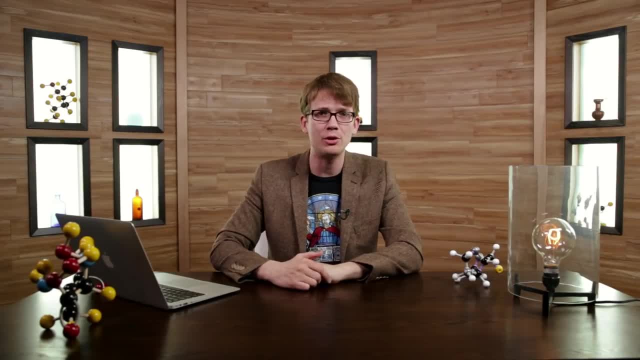 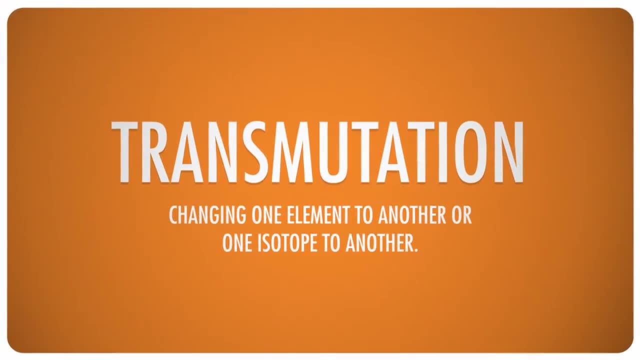 neutrons are isotopes, So changes in the number of neutrons in an atom create different isotopes of the same element. Both of these kinds of changes- changing one element to another or changing one isotope to another- are known as transmutation, And it is indeed possible. 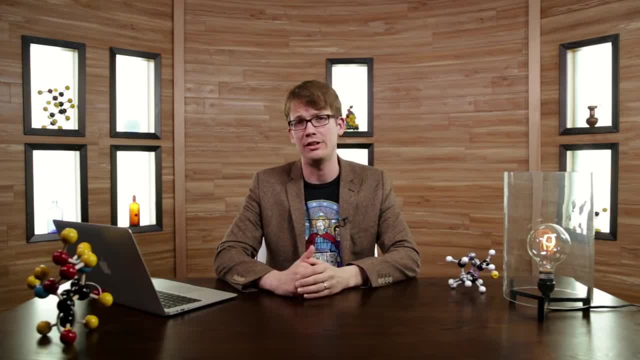 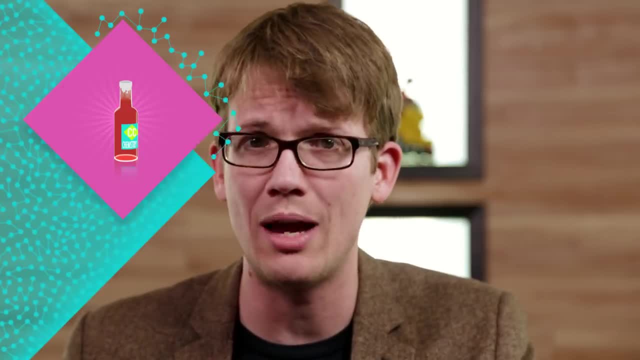 to transmute lead to gold. It's just so ridiculously expensive that the tiny amounts of gold produced could never pay for the process. But the very fact that it is possible should clue you in that nuclear chemistry is an entirely different flavor of chemistry sauce, Though, as with 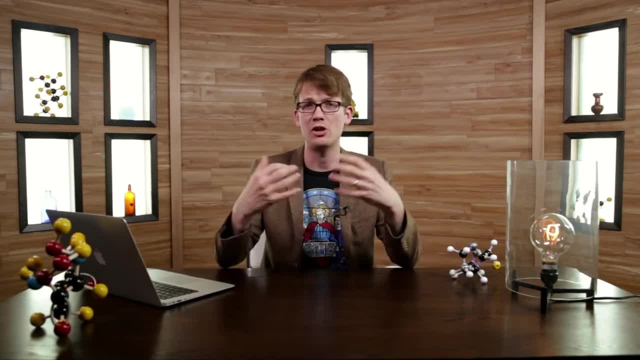 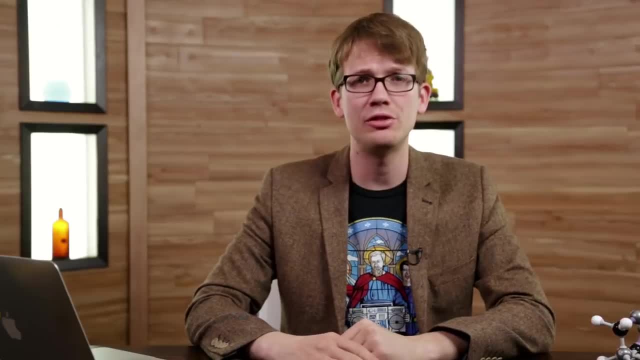 non-nuclear chemistry. the changes that take place in a nuclear reaction all come down to the atom's design. There's a desire to have what we all want in life: stability. Just as atoms are most stable when their outermost electron orbitals are full of electrons, certain combinations 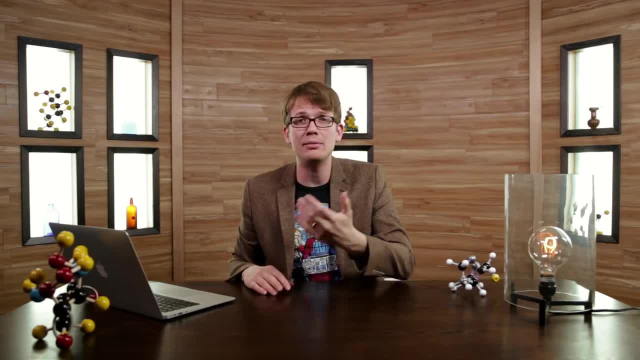 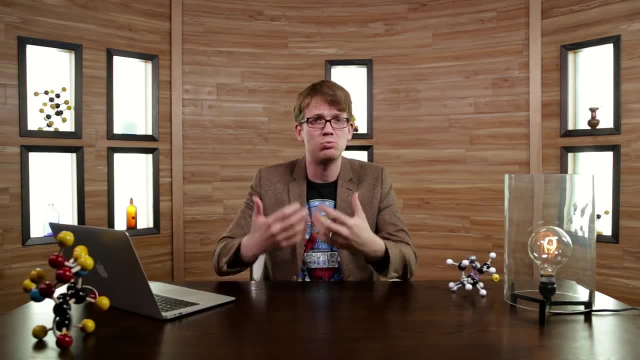 of protons and neutrons make the nucleus more stable And, just like when an atom gains or loses or shares electrons to stabilize its outer shell, when the numbers of protons and neutrons aren't ideal, the nucleus releases some of them to try to reach a stable configuration. 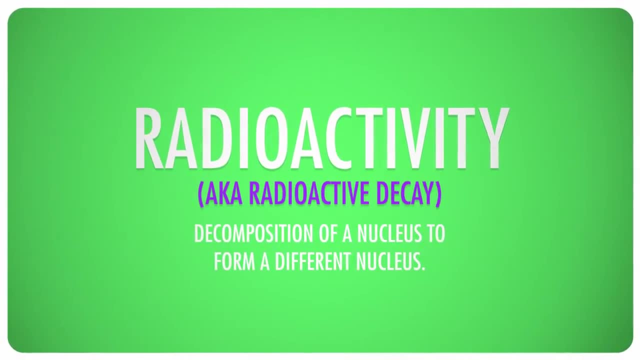 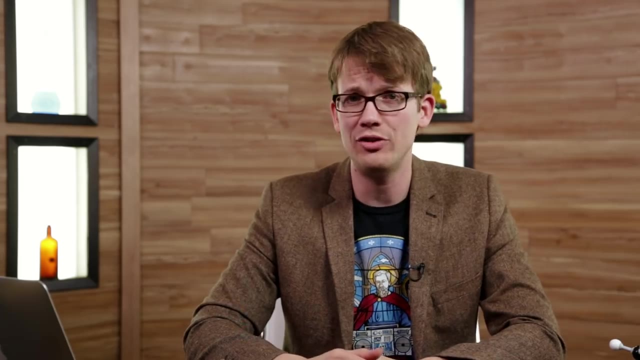 When a nucleus decomposes in this way to form a different nucleus, that's radioactive decay And, just like with other chemical reactions we've talked about, we need to know more about a nuclear reaction than just what's reacting and what's being produced. Probably 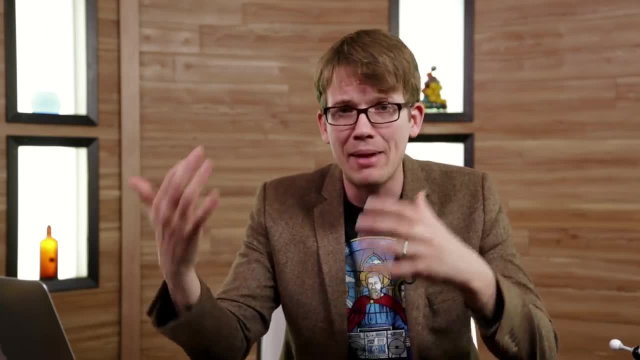 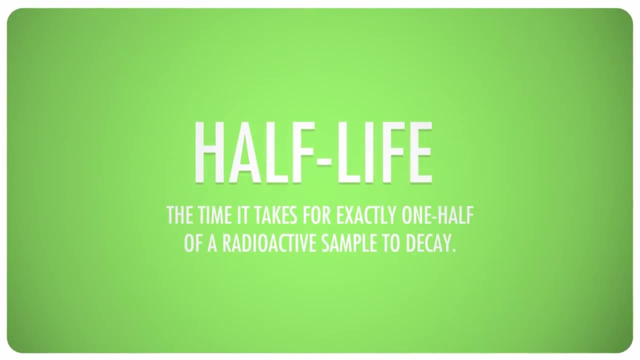 the most important thing to learn is how much of the product is being made and how fast. Now you've heard of half-life. It's the measurement that tells us just that: the time it takes for exactly one half of the sample to decay. 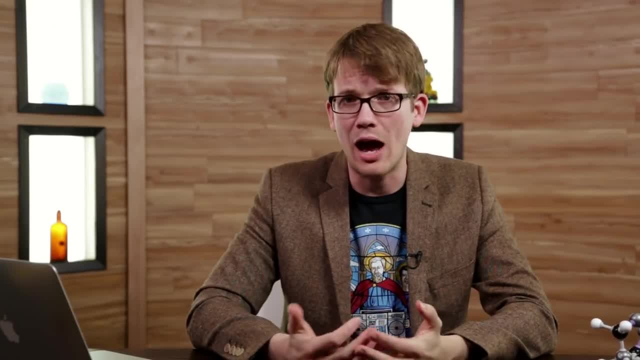 Different nuclei have different half-lives. By knowing the half-life, we can calculate how much of a sample will be gone in a given amount of time. For example, the half-life of phosphorus-32 is 14.3 days. That's exactly what we need to know about the half-life of phosphorus-32.. 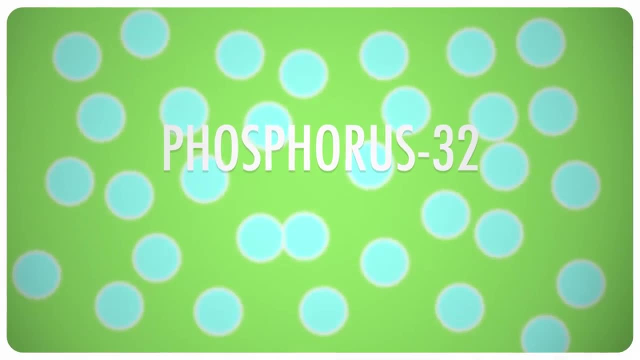 The half-life of phosphorus-32 is 14.3 days. That's exactly what we need to know about the half-life of phosphorus-32.. The half-life of phosphorus-32 is 14.3 days, So if you start with a 100 gram sample, after about two weeks you'll have 50 grams left. 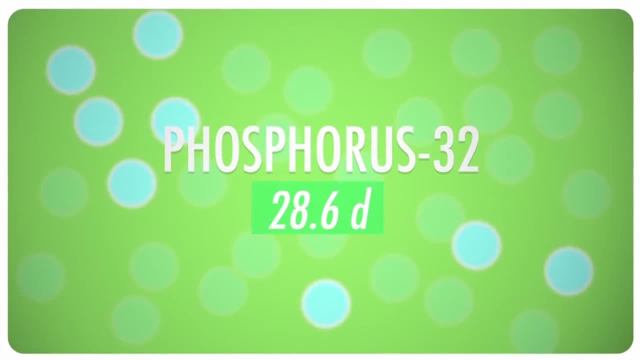 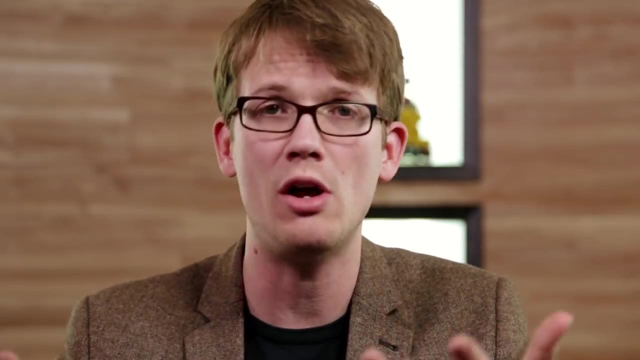 After another two weeks, half of the remainder would decay, leaving only 25 grams of undecayed phosphorus and so on. Now you might be asking: if radioactive elements are always decaying into more and more stable isotopes that are eventually no longer radioactive, why are they still around at all? Fascinating question. You seem to have brought your clever pants today. Well, it's fairly simple. Given enough time, all radioactive elements would decay into non-radioactive forms. Even ultra-stable bismuth would decay. Even ultra-stable bismuth would decay. 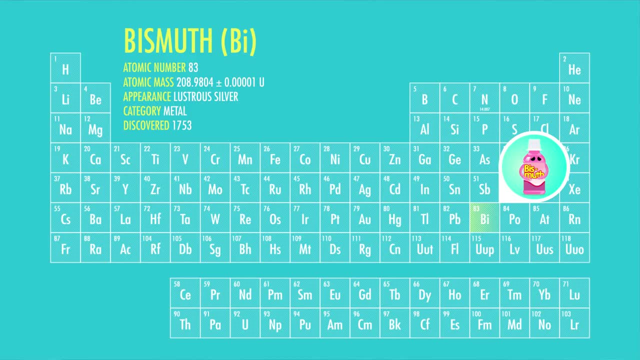 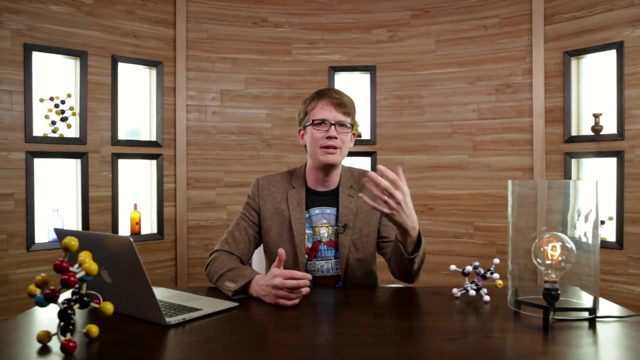 Even ultra-stable bismuth would decay With its half-life longer than the age of the universe. But elements with short half-lives are around because they were decayed into by elements that recently decayed into them The chain of decay from the elements originally produced in whatever supernova created them. 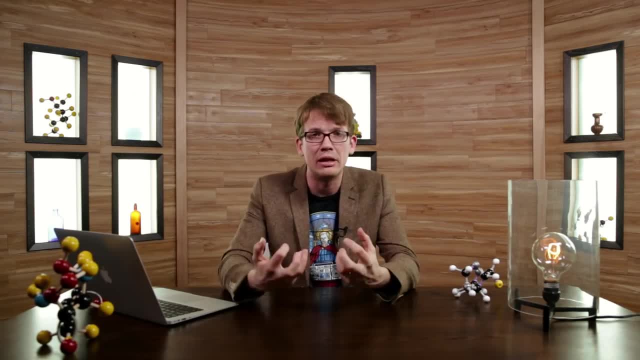 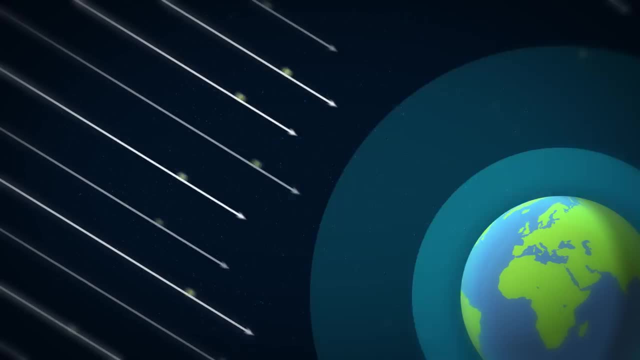 to the elements that exist on Earth now last billions and billions of years, Although I should note that some radioactive isotopes like carbon-14 in the atmosphere are constantly being renewed by cosmic rays. Now, radioactive decay occurs when a nucleus has a higher energy level than a potentially 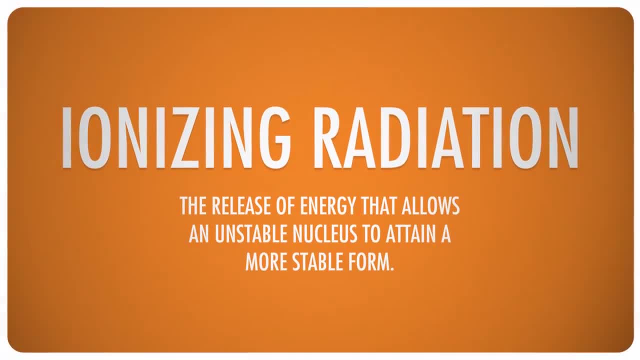 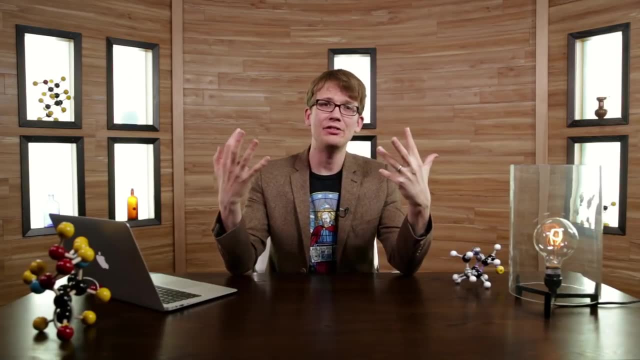 more stable version. Specifically, this difference in energy is released as what's called ionizing radiation, which you know as radioactivity. It's ionizing because it has enough energy to knock electrons out or add electrons to other atoms, essentially creating ions. 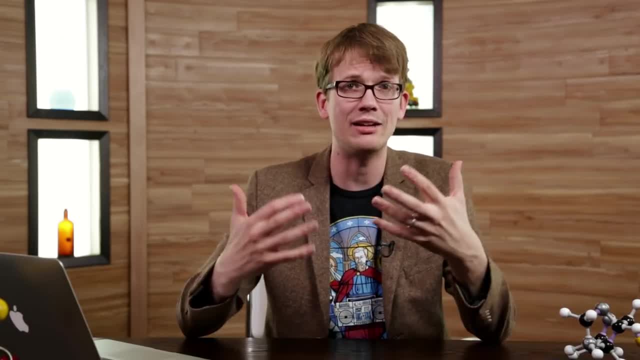 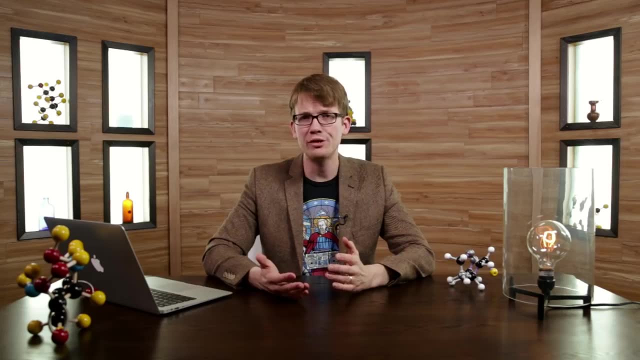 There are three general types of radioactive decay, each named for exactly what is released from the nucleus as it decays. Let's take a look at what may be the most famous radioactive element: uranium. By far the most common naturally occurring form of uranium is the isotope uranium-238.. 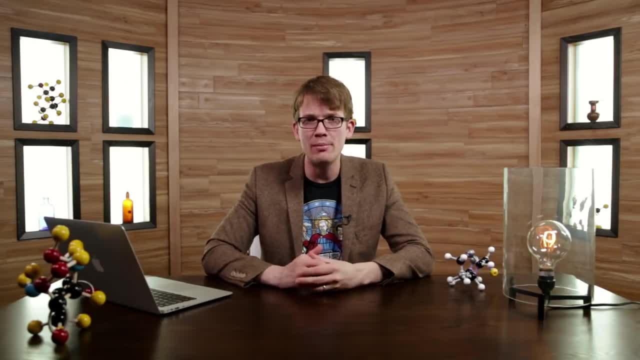 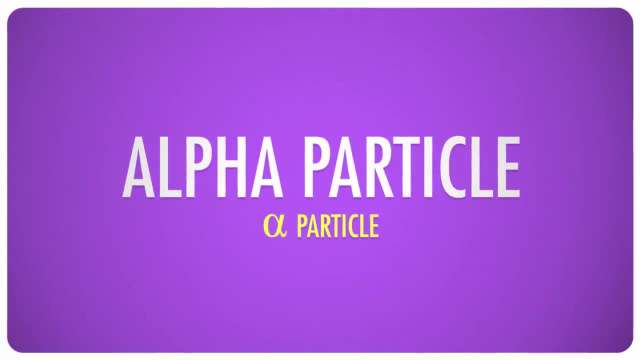 More than 99% of the natural uranium in the world is in this form. U-238 spontaneously decays into thorium-234 in a process that releases something called an alpha particle. This is called alpha decay, and the particle that it emits is basically the same as a helium. 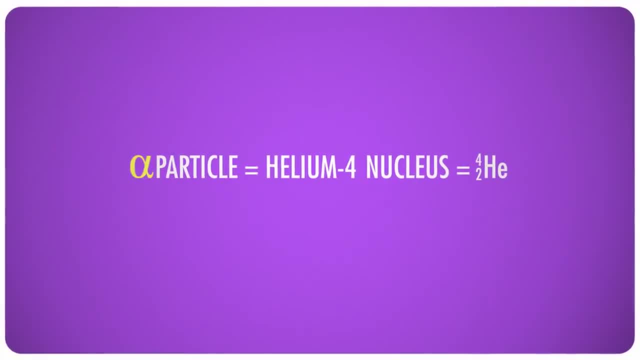 nucleus, two protons and two neutrons. We even describe it that way when writing it. So right away you can see that the math checks out. when it comes to the protons and neutrons, 92 minus 2 is 90.. 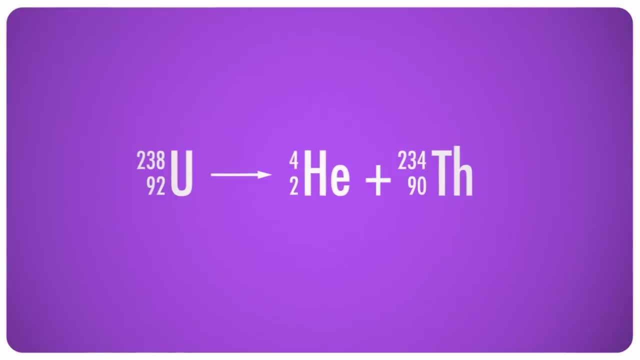 And 238 minus 4 leaves you with 234.. But you'll note that we don't write the charges. The helium nucleus obviously has a plus-two charge, and the thorium atom would have a negative charge as well. While it's not incorrect to write them, these charges are often emitted to emphasize what's. 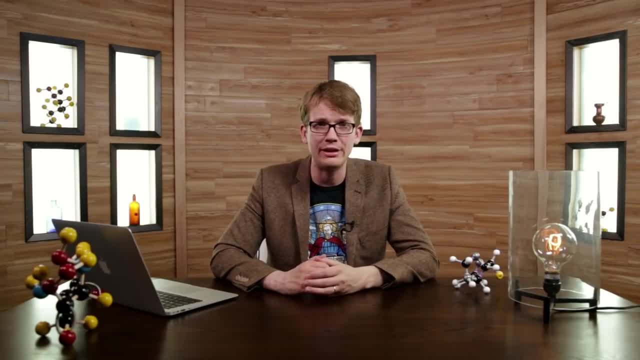 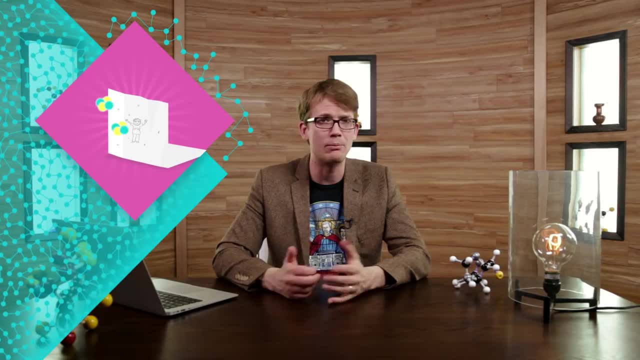 going on in the nucleus. Now, alpha particles have relatively low energy. they're pretty heavy as particles go, So while I try not to make a habit of walking around with a hunk of uranium in my pocket, alpha particles can be stopped by nothing more than a sheet of paper or cloth. 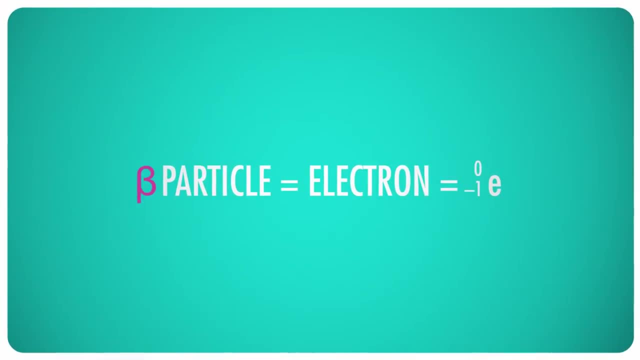 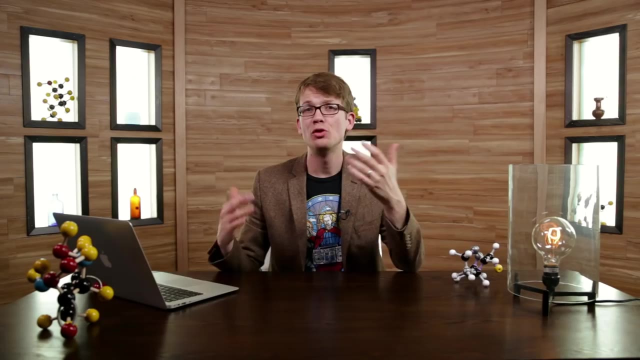 The second type of radioactive decay is beta decay, which simply emits electrons. It has somewhat higher energy than alpha radiation, But it can still be stopped by a sheet of aluminum foil or even the top layers of your skin, So that thorium-234 that formed when uranium underwent alpha decay. 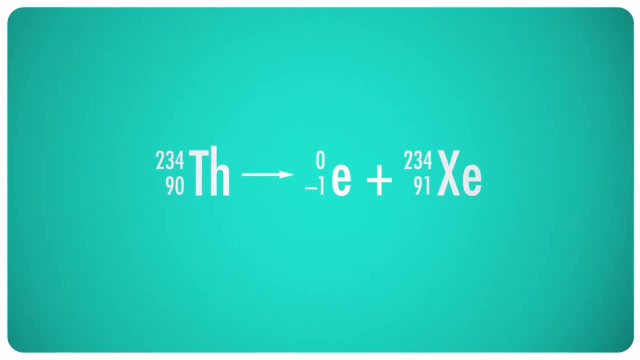 It can continue to decay on its own, and when it does, it undergoes beta decay, releasing an electron and an atom of xenon. Notice that, again, the way we write this is a little different. Even though the thorium emits an electron, we don't use the usual symbol for electrons. 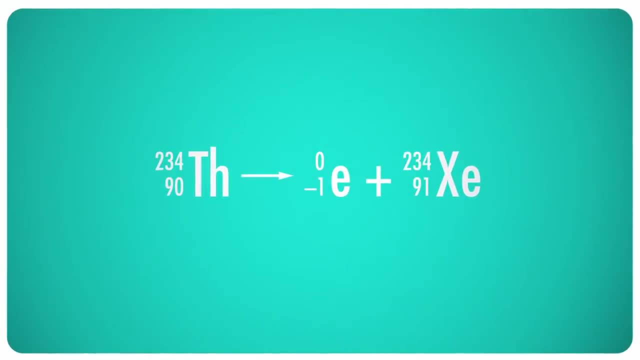 Instead we write it in nuclear notation form with the mass number at the top and the atomic number at the bottom. Since it's an electron and not a proton, we put a negative one for the atomic number. That probably seems a little bit weird right now, but next week, when we talk about nuclear, 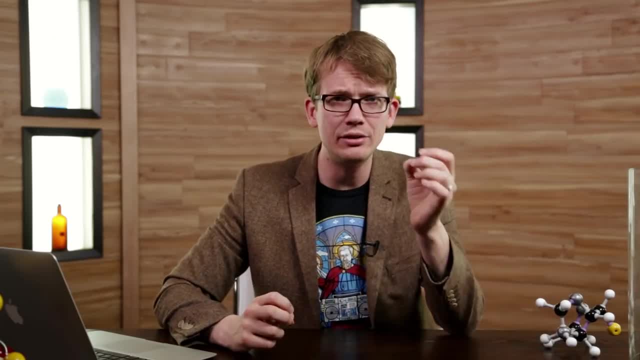 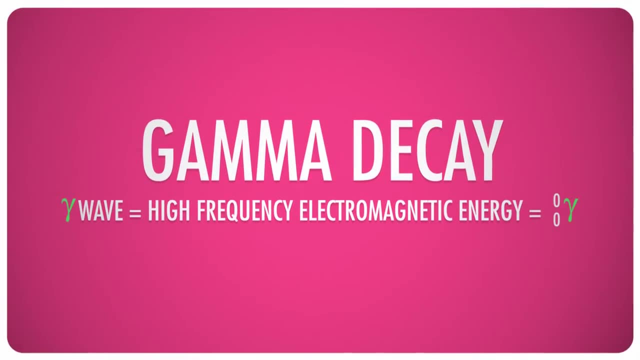 equations, you will see why it is useful. The third type of decay is a little different because it only emits energy, not a particle. It's called gamma decay and it releases electromagnetic radiation similar to visible light or UV radiation, but higher on the energy scale. 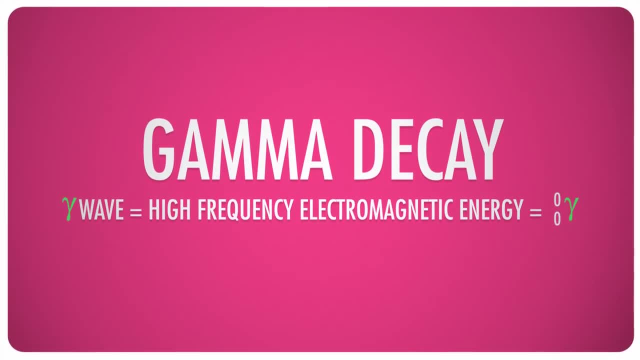 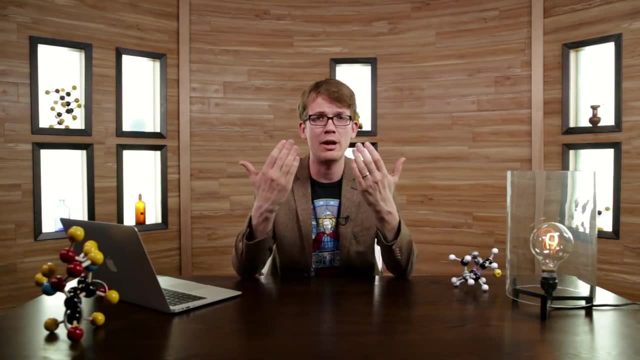 Because it's just energy. gamma radiation has no mass and contains no protons, neutrons or electrons, So it's written with two zeroes. This form of radiation is often released when electrons transition from an unstable, excited state to a more stable state that has a lower energy. 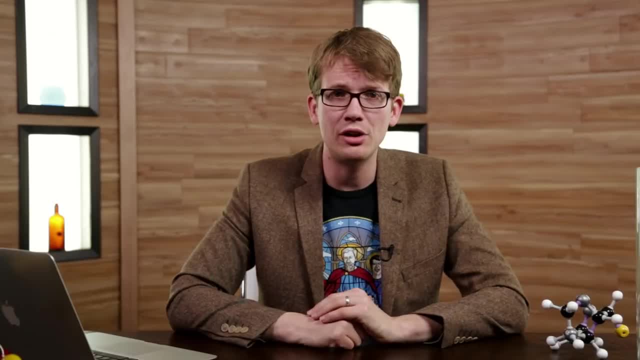 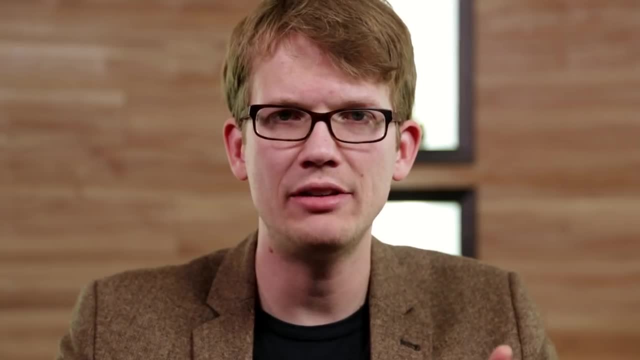 That's called the ground state. Depending on how much energy the electron loses, the extra energy can be released in the form of visible or ultraviolet light, x-rays or gamma waves. Let's take the example of nickel-60.. Imagine there's an atom of nickel-60 with one or more of its electrons in an excited 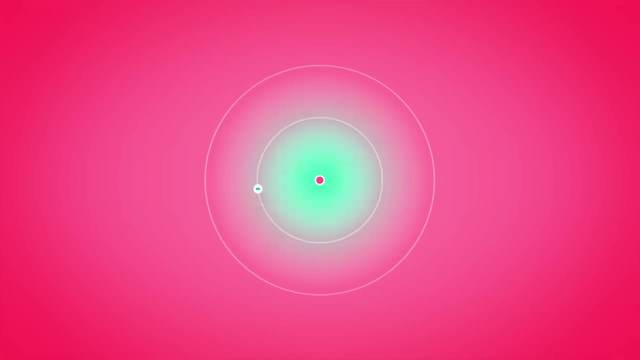 state. That's what the little asterisk designates. Atoms can get to this state when they are the most stable, So it's written with two zeros. The electrons are the products of radioactive decay or if they get bombarded with radiation. 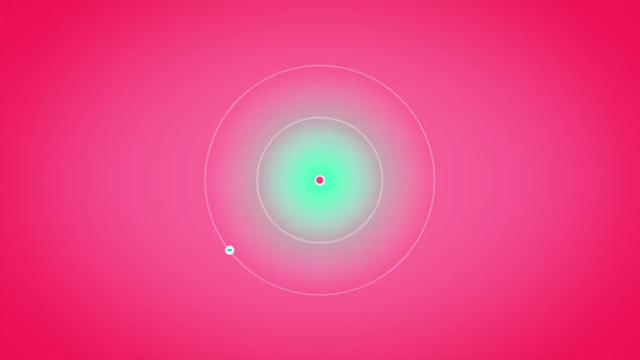 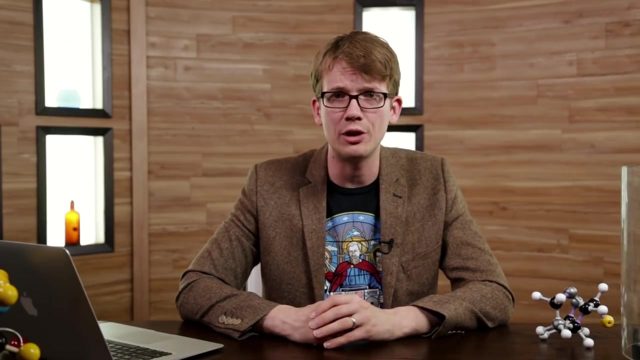 from other reactions, pushing their electrons into a higher energy level. Now, when all those electrons drop down to the ground state that atom is going to release some gamma radiation. But this kind of transition can also take place where other kinds of nuclear reactions are going on. 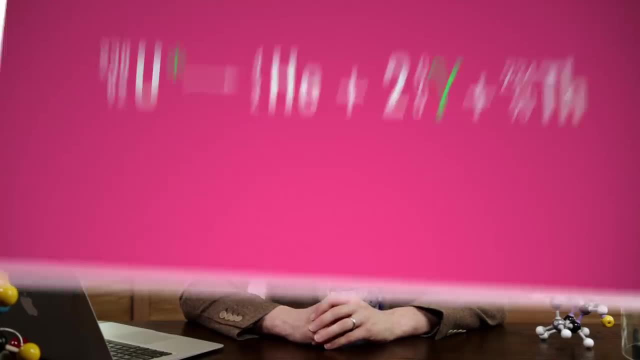 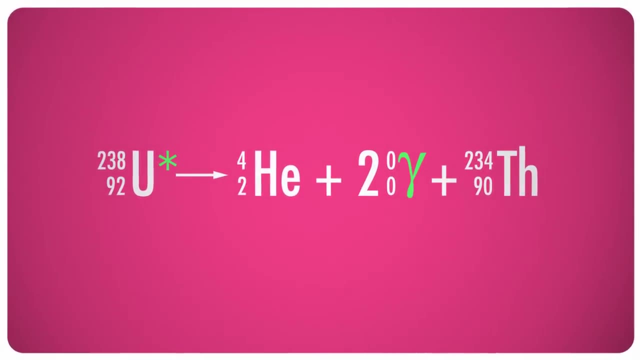 So gamma decay often occurs along with some other form of decay too. So, for example, if that uranium atom is in an excited state, when it decays into thorium, it can simultaneously release gamma waves as well as the alpha particle I already mentioned. 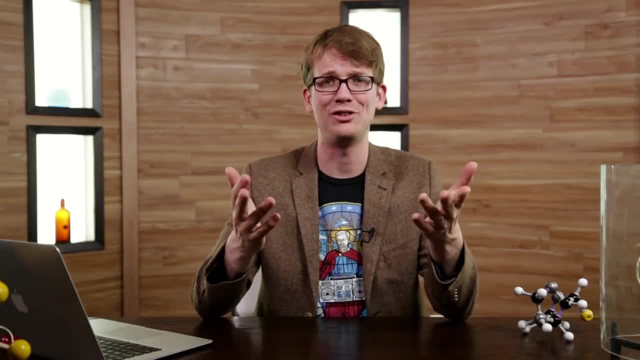 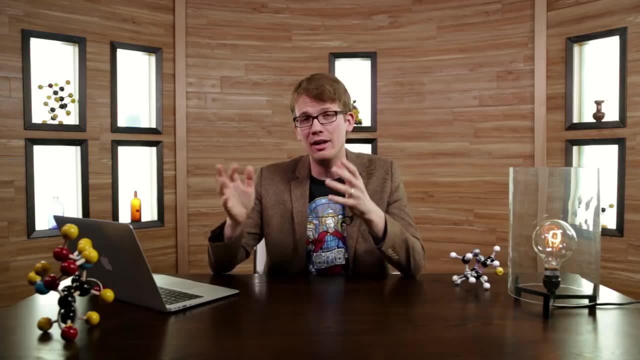 Now you might have heard of gamma radiation more than the other term, And I'm not saying the other kinds of mention, because it can actually do some serious harm, like potentially turning you into a giant green rage monster that doesn't obey the laws of conservation of matter. 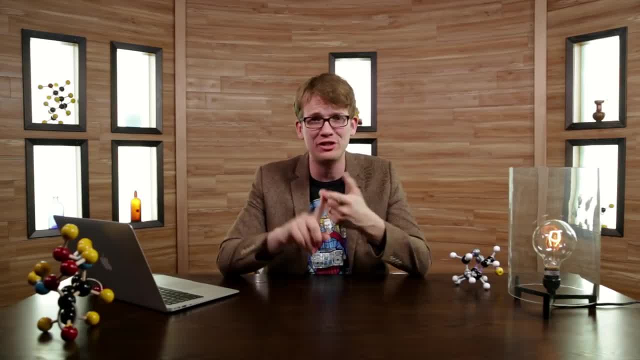 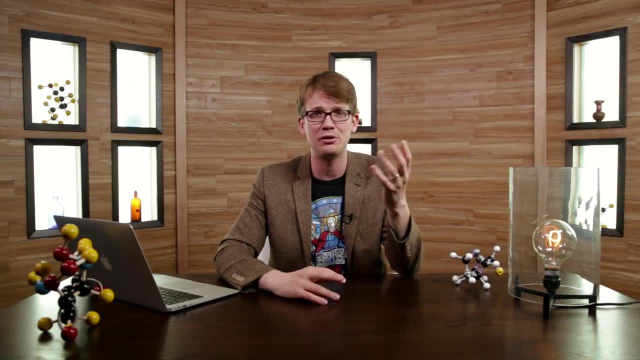 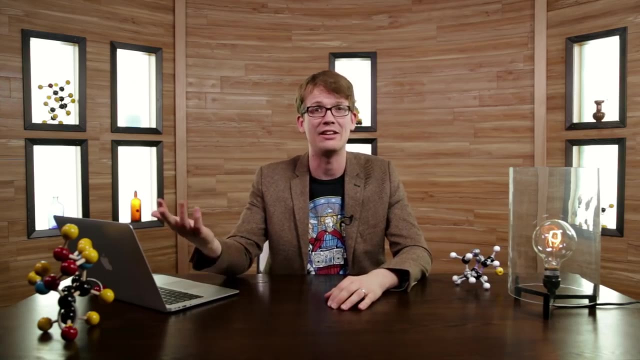 Unlike the particles emitted by other kinds of radiation, gamma rays can penetrate your skin, your cell membranes and, ultimately, the organelles within your cells. So gamma radiation can not only cause skin burns, nausea- other symptoms we associate with radiation poisoning. it can also alter your DNA, causing mutations and cancer. Okay, but to turn the frown upside down, there's one more type of radioactivity that, I am happy to say, is really simple. It's called spontaneous fission, and it occurs when an atom simply breaks into two smaller atoms without any outside help. 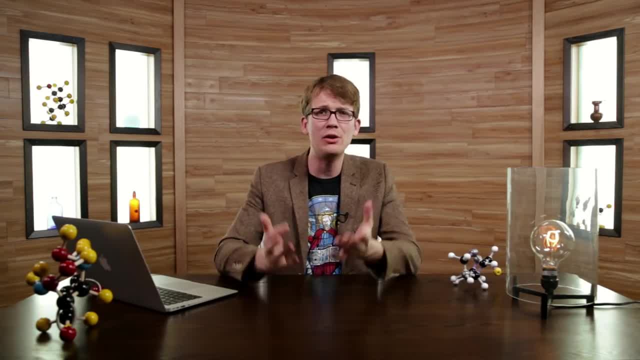 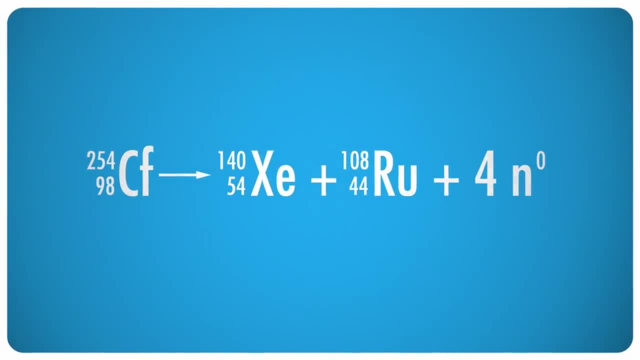 This occurs at a ridiculously slow rate in most cases. In fact, the only substance that does it at a rate that's sufficient to serve any purpose is californium-254,, and that purpose is to produce neutrons for use in other nuclear reactions. 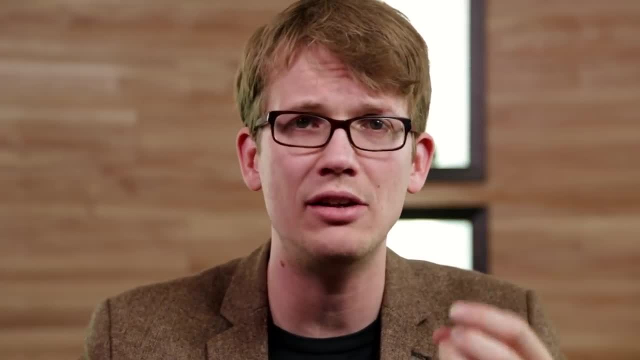 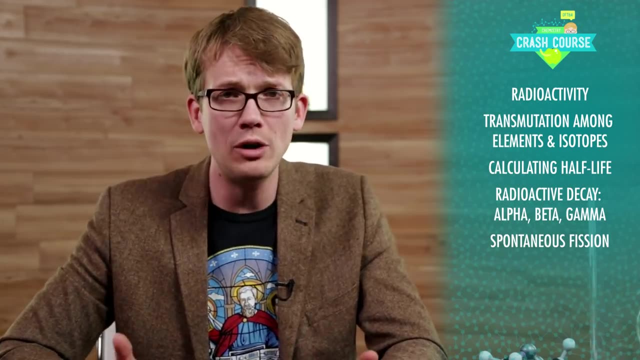 But we'll talk more about that when we go into fission fusion and how scientists use and control nuclear reactions. In the meantime, thank you for watching this episode of Chronicles. If you listened carefully, you learned what radioactivity really is and about transmutation. 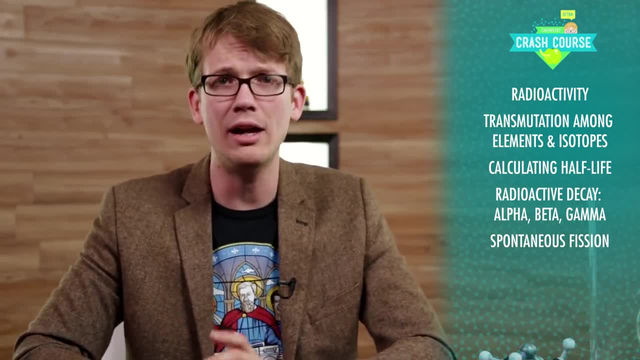 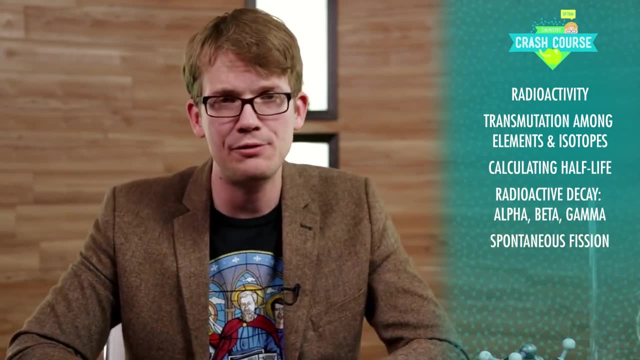 among elements and among isotopes, and how to make calculations based on an element's half-life. You also learned about different types of radioactive decay- alpha, beta and gamma- and about spontaneous fission. This episode was written by Ida Gonzalez and Blake DePastino. 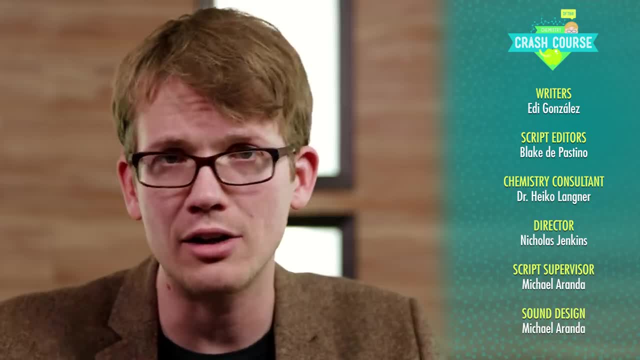 It was edited by Blake DePastino and our chemistry consultant is Dr Heiko Langner. It was filmed, edited and directed by Nicholas Jenkins. The script supervisor was Michael Aranda, who is also our sound designer and our graphics. team is Thought Cafe.